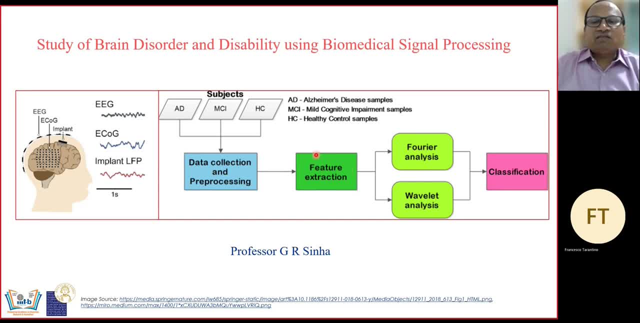 And once the feature sets are finalized, those are converted into feature vectors and the feature vectors are then subjected to a number of other tools. And finally, we classify the data and we analyze whether the data is of Alzheimer's person, Alzheimer affected person, whether the data is of mild cognitive impairment subject or the data is of healthy person. 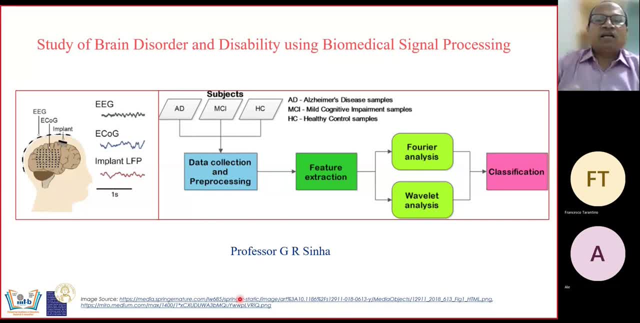 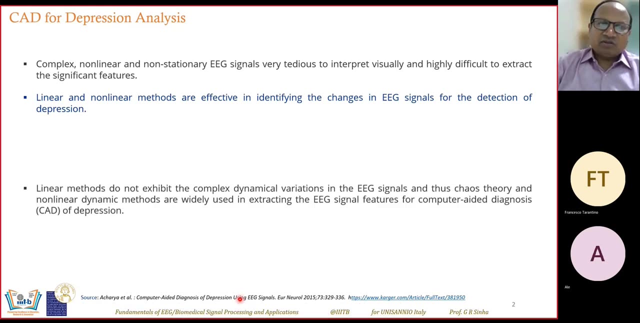 Okay, Or a healthy subject. So that is the general purpose: understanding and signal processing flow, especially the biomedical signal processing which is essentially used to analyze the other different disorders and disabilities. So this was the- you know a few slides where I was a little fast in the previous lecture. 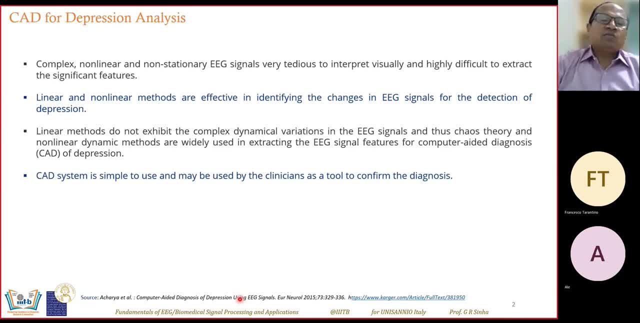 So let's just do three more, two, three more slides, which we had already covered in the previous lecture, and then continue. So we generally use computer-aided diagnosis for a depression and disorder analysis. We can have any kind of system, any kind of method that can be provided by the computer-aided diagnosis system. 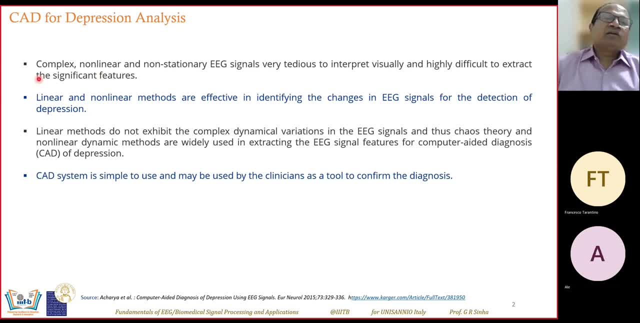 We know that EEG signals are complex in nature, They are generally nonlinear and non-stationary and therefore understanding and interpreting the EEG signal is extremely difficult task. So therefore, a number of methods, Either linear, nonlinear methods, are available. Linear methods generally do not exhibit the complex dynamic variations because the basic nature of EEG signal is complex and nonlinear. 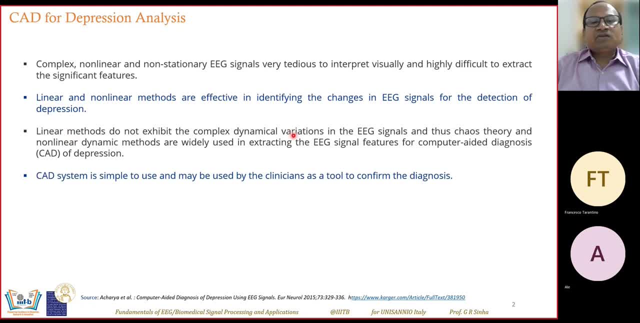 So when we choose linear method for analysis, the dynamic variation and dynamic characteristics of EEG signal might not be interpreted very well, And the chaos theory and the nonlinear dynamic methods Therefore are recommended as better methods for extracting the suitable EEG signal features. And those features are used by the computer-aided diagnosis in order to study different kinds of depression and disabilities. 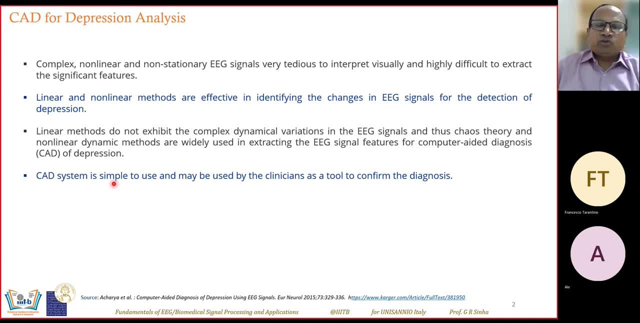 So the CAD system is simple to use. where other different stages will be there, all stages will be automated stages inbuilt with the different mRNAAi models And the clinicians and the radiologists at MIT- everybody are running these different objectives in mijn models. 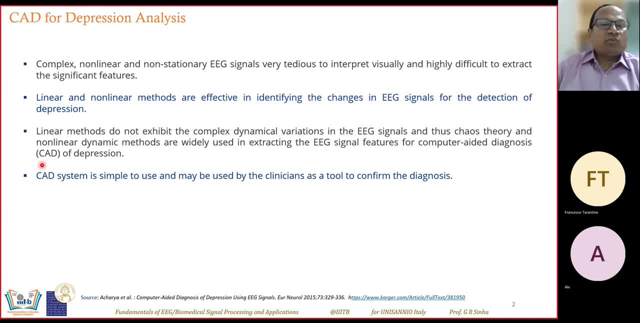 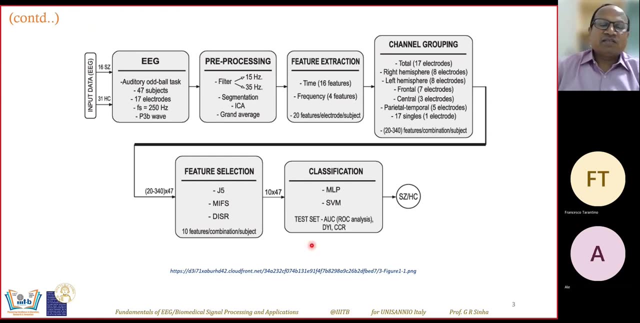 Thank you very much. physiologist, or the physicians, can actually work with the CAD system very effectively and comfortably and that CAD system can help them in their diagnosis and treatment process. So this is under purpose. you know the diagram where you can say: this is a CAD. 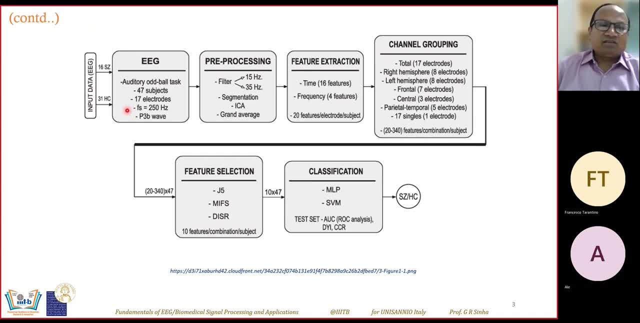 where the data input is captured from a number of channels like EEG, and this may be ERP as well. When we use auditory oddball tasks or other paradigms- you have seen RC paradigm. there are different paradigms of the stimulators, So we can either have 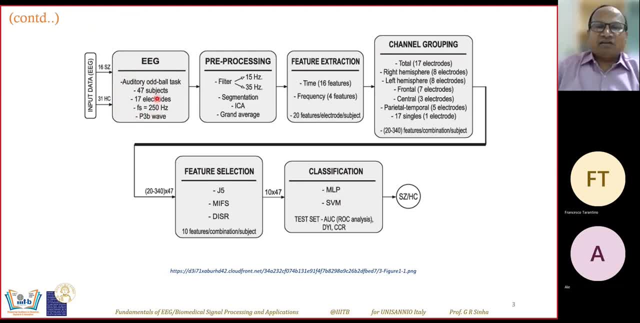 EEG or, you know, P300 ERP signals or EEG signals. So we take them to the pre-processing using suitable filter. The filter may provide the appropriate and the meaningful the signal, The signal which can be subjected to a different feature extraction method where you can extract. 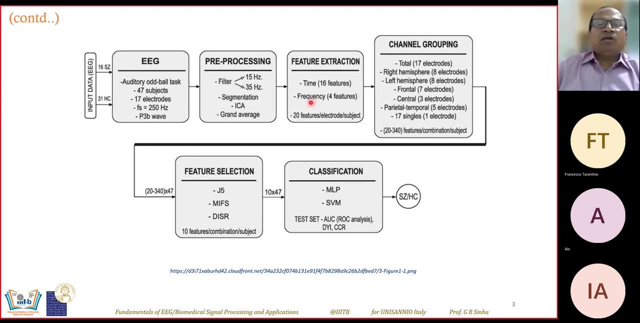 either time domain or frequency domain, or in both domain, we can extract the features. Similarly, you know, extracting the features, we can even group the different channels. and then, which are the channels which are bringing the information from frontal area? which are the channels which are bringing the information from central area or parietal area? 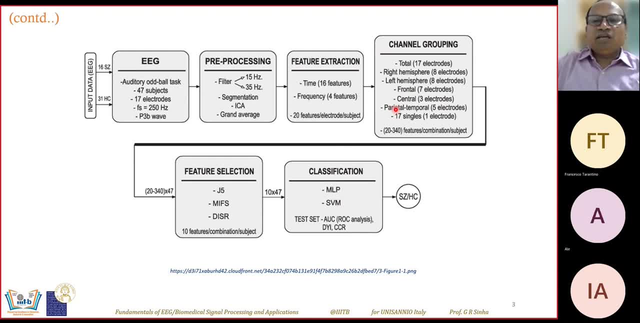 we can then decide which you know area is important for us, based on the application, And then appropriately, features are selected and then, using a suitable you know the classifiers, we actually classify the data into whether the candidate or a subject is suffering with. 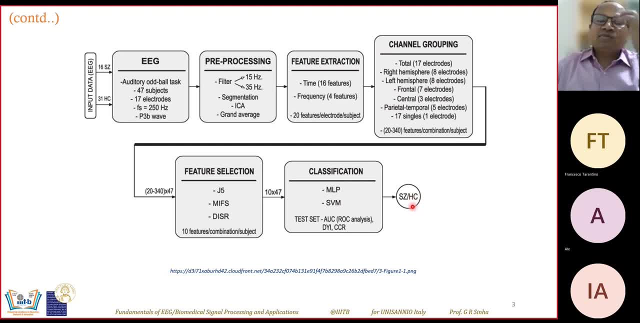 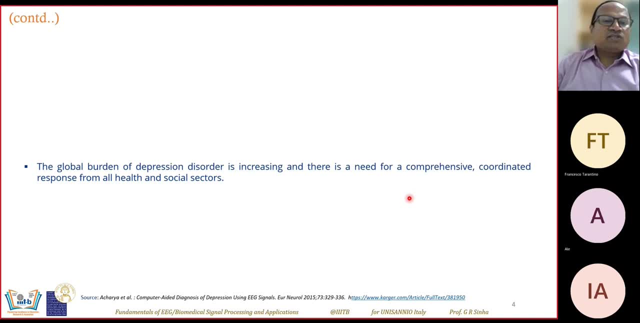 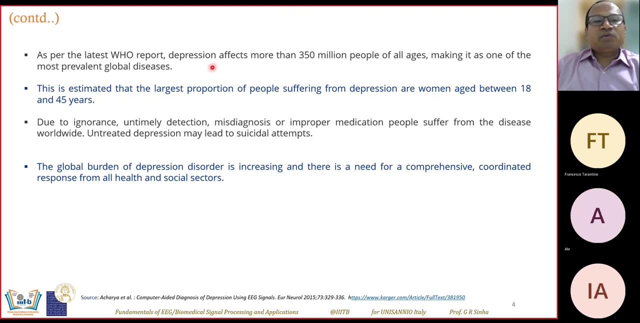 some depression, like schizophrenia or some Alzheimer's disease, or is a human, you know, a healthy person Or a healthy subject. So this is the approach where, if you remember last time, we were trying to understand this: the depression. as per WHO report, it affects more than 350 million people of all ages. because, 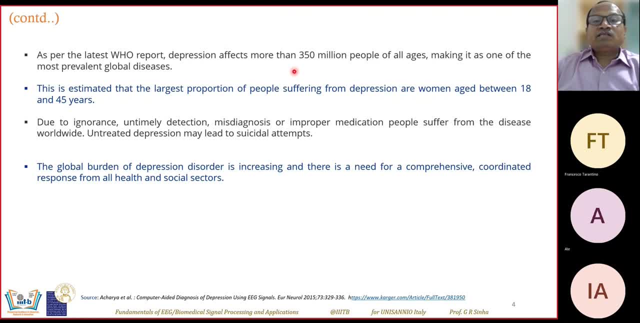 you are planning to do something on the psychology, So you need to understand this. You know the psychological impact is also a factor that causes a depression, like during COVID-19.. The pandemic, You know, lot of impact was psychological impact. because of that uh, you know, thousands of people uh went. 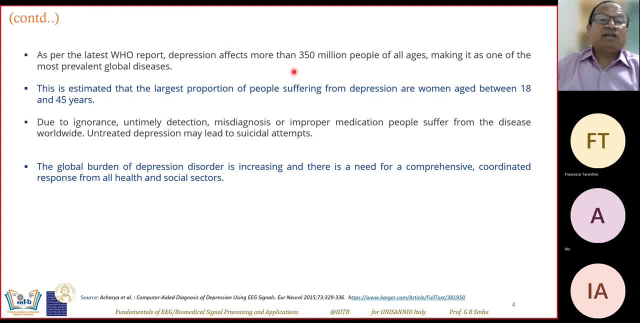 through, uh you know, uh, the the depression and stress stages. so 350 million people are especially, uh, you know, of all the ages, uh, you know the depression affects these number of people, making it as one of the most prevalent global disease. this is estimated the large, largest. 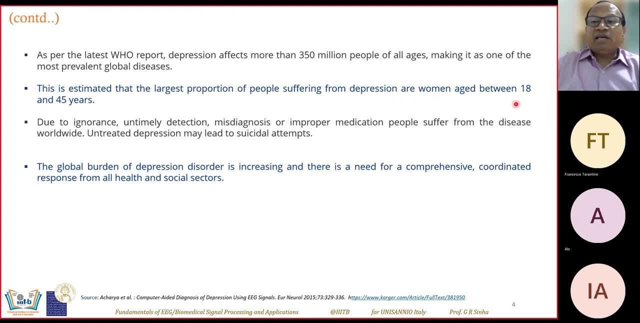 population of people suffering from depression are women aged between 18 and 45 years, so you can see that a lot of young women, a lot of adult and young women are also suffering with the depression due to the ignorance. many people simply ignore that there is nothing, like you know the depression. 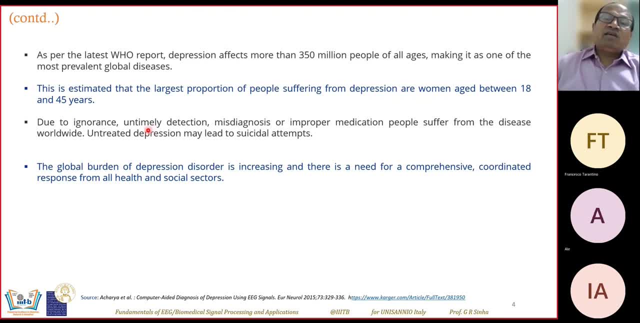 as a disease, depression as a disorder. untimely detection is there. they don't actually go for the screening, go for the test and therefore misdiagnoses or improper medication. people suffer from the disease worldwide. untreated depression may lead to suicidal attempts- also so suicidal, you know- attempt. 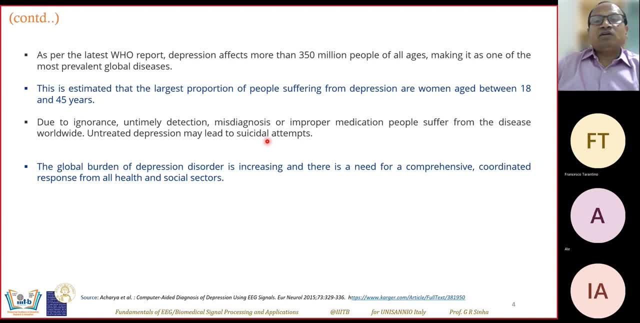 is nothing but a psychological impact, where the person undergoes, uh, undergoes with uh, you know, very much negativity and negative psychological impact and person decides to, you know, commit suicide. so the global burden of depression disorder is increasing and there is a need for compression and there is a need for a more comprehensive, coordinated effort, coordinated response from all. 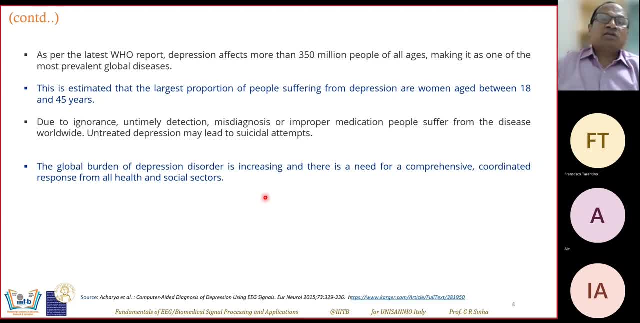 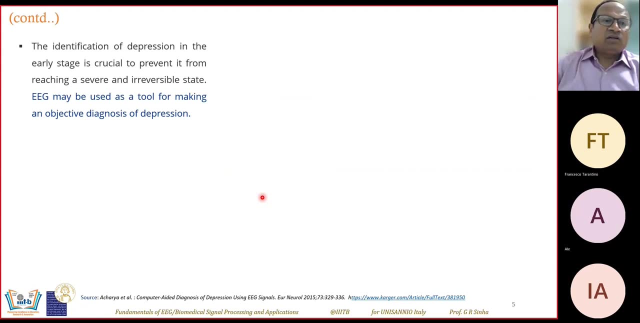 these stakeholders, either from health care or the social sector, the, the counselors, the psychologists, psychotherapists and the people who are involved in a number of mindful practices which could help the people to recover from various psychological disorders. so, uh, the identification of depression in the early stage is therefore very important. so what we can do is we can start to look at the 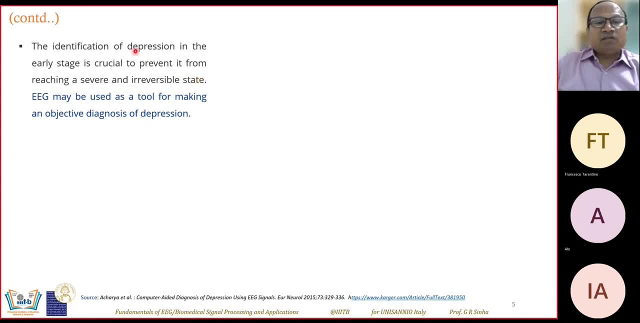 different stages of depression, so that one's life can be saved, and the that other disease can be diagnosed are reaching, so that it cannot reach to severe and irreversible state. you have seen that in our previous lectures we have talked about bci, we have talked about biomedical signal processing. 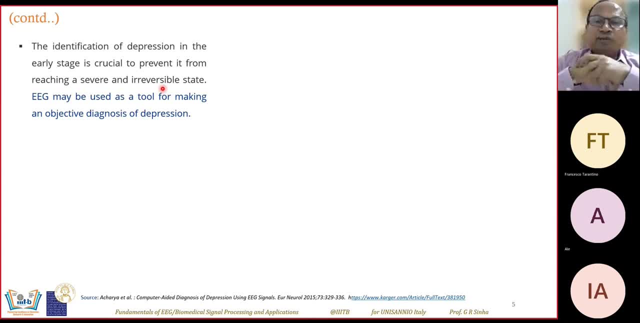 where we know it very well, a neurofeedback signal can be generated in the form of auditory signal, in the form of picture or in the form of tactile signal, so that the bio-medical signal can be, that can even attempt to reverse the problem, in the form of feedback signal which is given back. 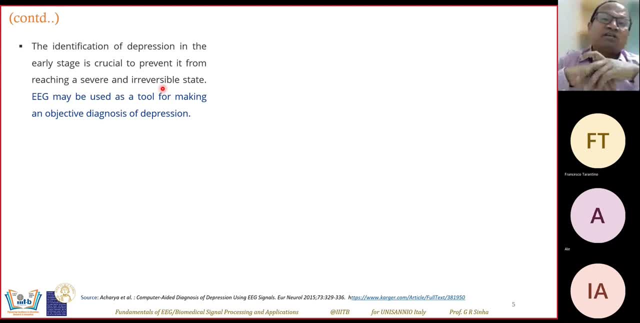 to the brain signal, So that can only work when the problem is detected at early stage. Otherwise, you know, when it is very late, when it has become critical, it's very difficult to diagnose and prevent. So EEG may be used as a tool for making objective diagnosis of depression. 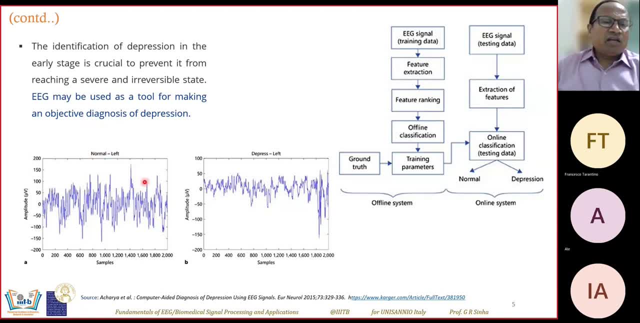 These are some diagrams where the normal lip- you know the lip brain EEG signal when the case is normal and when the case is abnormal. you see the variation in the EEG signal And we know all the natures related to alpha, beta, gamma, theta and beta And based on the 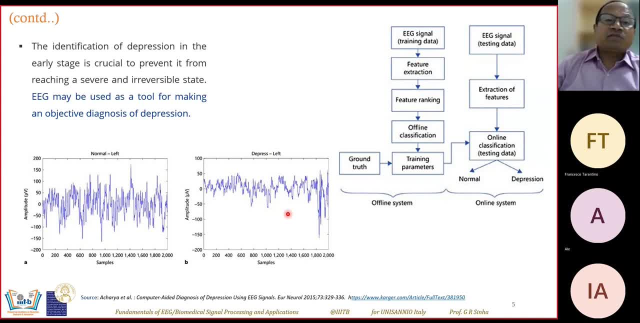 normal waves or waves, you know, brain waves of all the normal persons and subjects. comparatively, it can be analyzed and it could be, you know, decided. Determine that what could be the cause of the variation in the EEG pattern of the waves and 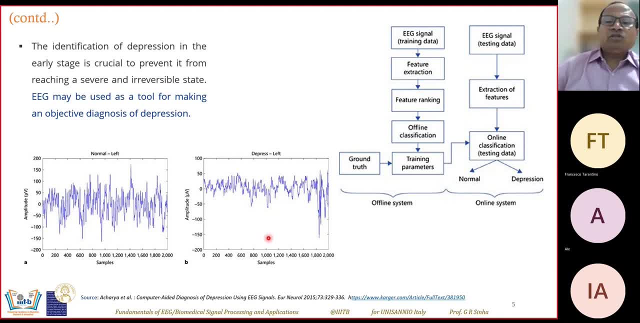 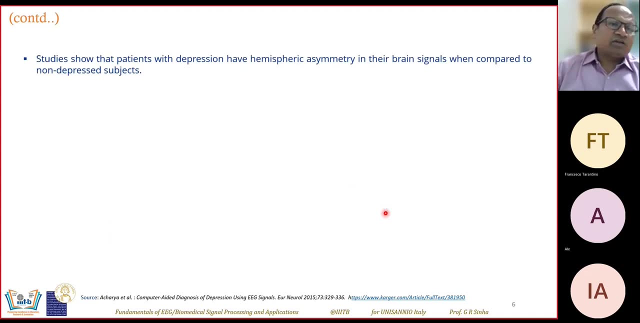 accordingly. you know detection can happen. So the you know this is a general purpose diagram. I do not need to repeat that there are two stages: training and testing stages, which are used in detecting the and treatment of the brain disease and disorder. 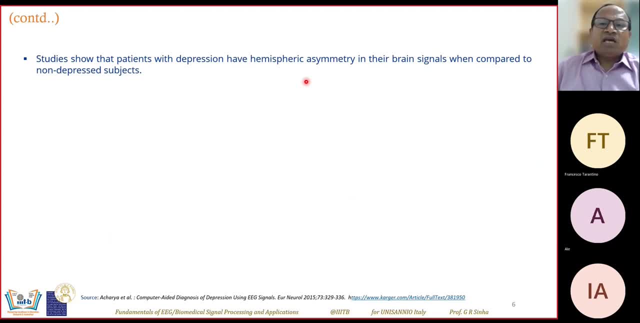 And there are studies that report that patients with the depression have hemispheric- actually- asymmetry. They are brain signal. Hemispheric asymmetry is found in the brain signal in comparison with non-depressed subject. So whenever you go to a particular person there, 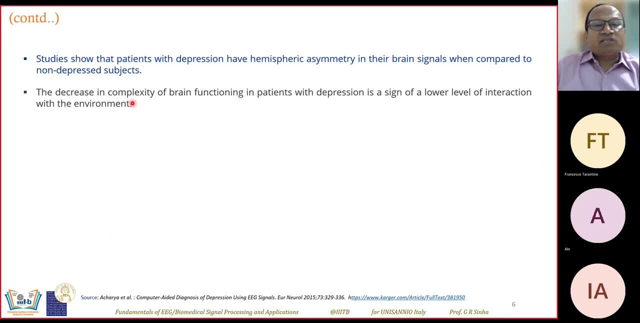 the signals will have the asymmetry. The decrease in complexity of brain functioning in patients with the depression is sign of lower level of interaction with the environment. So when you find that there is a decrease in the complexity in general, you know that the brain functionality 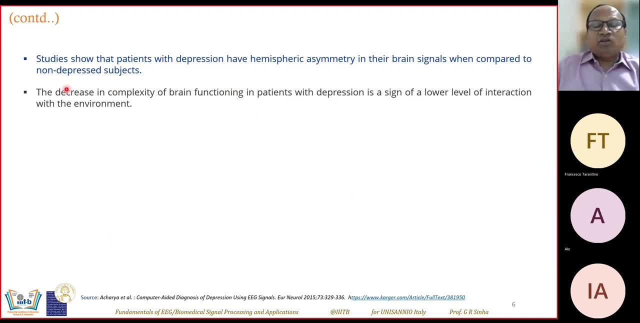 is very complex, But if there is any decrease in, you know there is any decrease, that s a sign of depression and actually lowers the level of interaction with the environment. The subject or a patient who is suffering with this difficulty, you know, always exhibits or expresses apprehension to be. 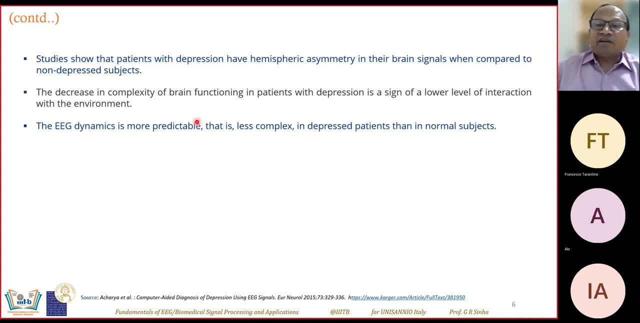 you know, mixing with or interacting with the environment, his friends, family and other people, EEG dynamics is more predictable and that is less complex as well. And in depressed patients, in a normal subject, the patient differs significantly in their dynamic response to the therapeutic interventions during first and the recurrent episode EEG signal asymmetry. 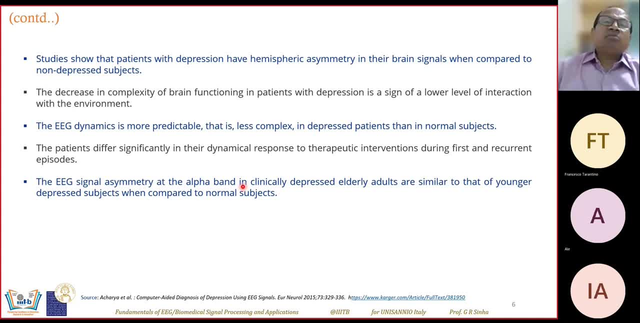 at the alpha band. this is what I was trying to tell you: that biomedical signal. where does it come into picture? EEG signal asymmetry, where it alpha band in clinically depressed elderly adults are similar to that of younger depressed subjects when compared to normal subjects. So this is. 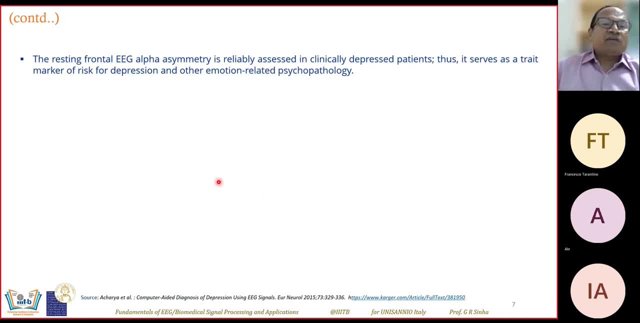 how one can predict the disability resting. frontal EEG alpha asymmetry is assessed in clinically depressed patients and it serves as a trademark of risk for depression and other emotion related psychotherapy difficulties. the increased variability of interior EEG symmetry. you know that there are different parts and from different part EEG signal is recorded and 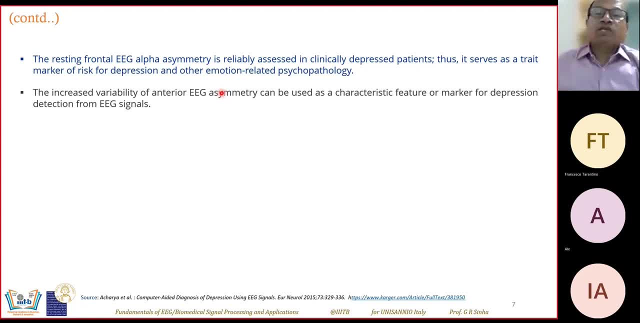 asymmetry is observed and based on that the conclusions are drawn. so this asymmetry can be used as a characteristic attribute or a marker for depression detection from the EEG signal, even though multiple courses of anti-depressant are used to treat individuals with the depression. but medication, you know to to what extent you will go for medication. so the relationship between 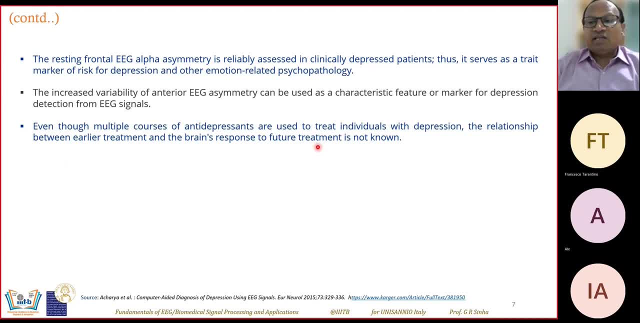 early treatment and brain's response to future treatment is generally not known. but yeah, at least the early treatment, the early detection can help the person to save the life. so a lot of medicines also affect the, the mental health, and the depression is one of the reason for that. also, the effects of drugs on EEG vary and are often dose dependent. how much 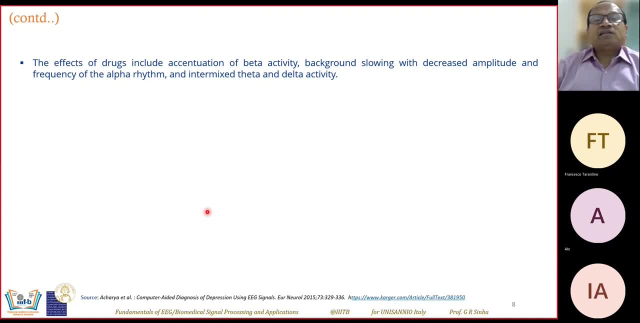 dose one can actually- you know, can- can tolerate and can sustain with the effects of drugs include accentuation of beta activity. so when there is an overdose of drug or the how does drug effects accentuation of beta activity is reported, background slowing and decreased amplitude and frequency of algorithm that is intermixed with theta and delta activity. 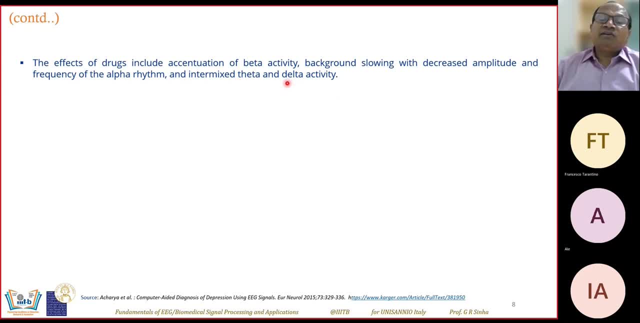 so this is how, with the help of beta, theta and delta activities- uh, the particular pattern- one can study the effect of drug in the person who is undergoing the depression disorder, the most common changes in EEG characteristics due to medication. so smoking benefits and elder AD, they can be found in smoking. 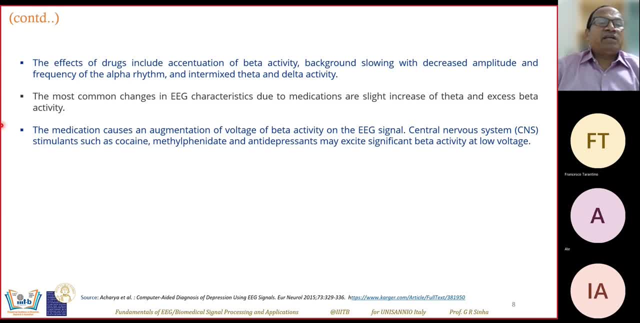 and belial drugs today by necessarily semaine action. here we strange. so there it is that you know high mandates are missing. there it is is doubtful for people to, especially long term, sebagai led to be completely independent in cancer and surgery in a phablet muscles absence. and Oriental engineering is required in such case, which also indicates showing significant, slight but very good increase of T and E creativity. so when a person is having, you know, more and more-medication, so that is indicated by very low, you know, slight, increase in the T activities but huge increase in the beta. 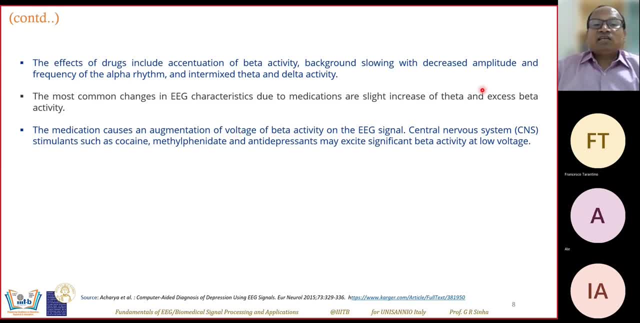 activities that can indicate that the person is taking a lot of medication and is causing depression in him. so medication causes an augmentation of voltage, beta activity: voltage of beta activity augmented. the beta activity increased. the beta activity- and this normal science increases. a little activity is augmented. Therefore, excess beta activities are reported. Central nervous system. 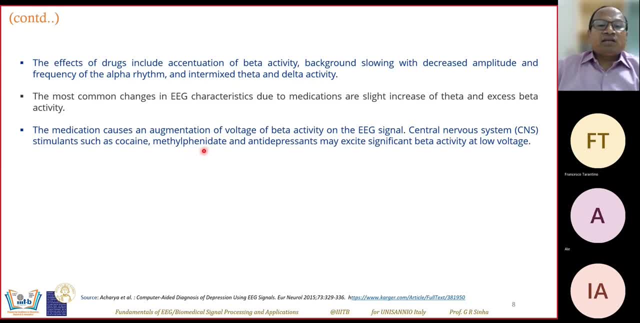 stimulus such as cocaine, metha, you know, methylphenidyl and the antidepressants may excite significant beta activity at low voltage. So these are all, cocaine and other things are, you know, considered as drugs or part of medication. even So, high doses of several 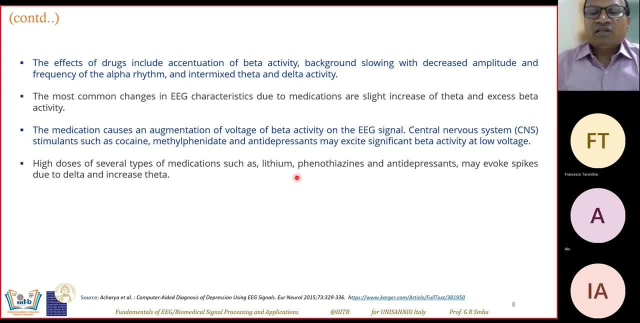 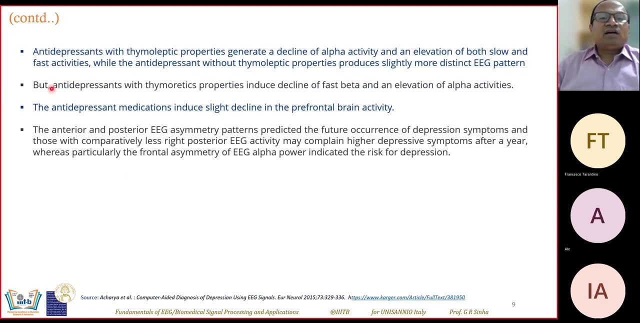 types of medications such as you know lithium, you know thiazines. antidepressants such as such kind of medications may evoke spikes due to delta and increase the theta as well. So antidepressants generate a decline of alpha activity and elevation of both slow and fast. 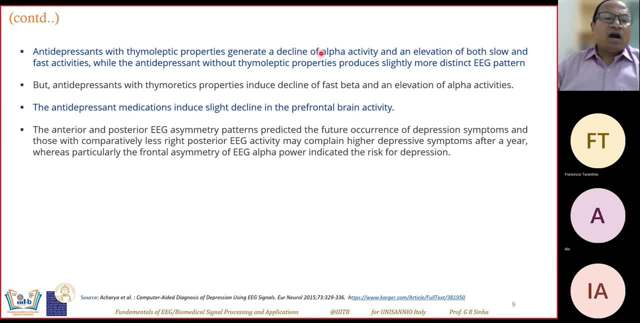 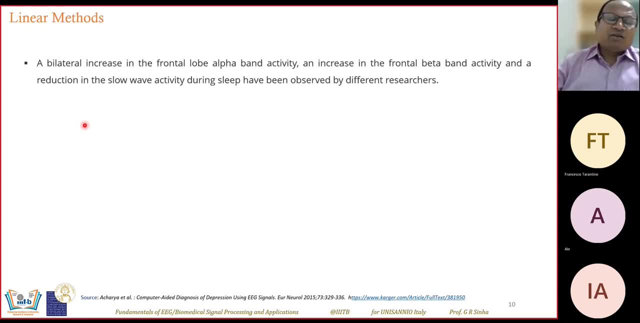 activities and so on. So we can understand. how does you know the medication impact different parts of the brain. So what are the methods which we were discussing about to study these disorders and disabilities? There are different types of methods, like linear method. 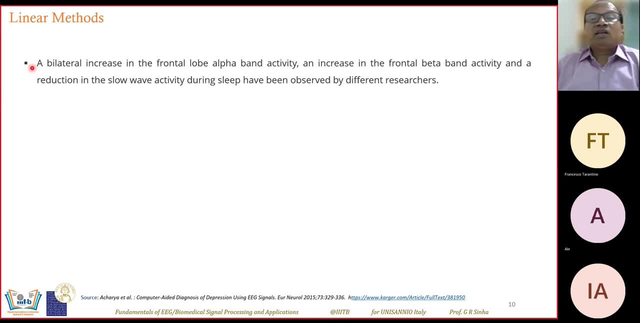 which is not considered as a good one. but linear methods can also be tested and can be used in order to study. So bilateral increase, bilateral increase in frontal lobe alpha band activity and increase in the frontal beta band activity and a reduction in slow and fast activity. So these are the methods which we were discussing about to study these disorders. So what are the methods which we were discussing about to study these disorders? So what are the methods which we were discussing about to study these disorders? So we can see that. 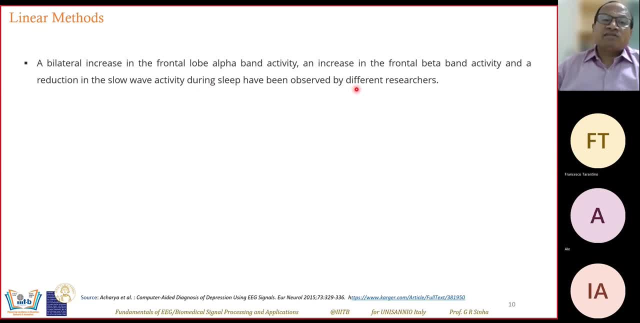 the slow wave activity during sleep have been observed by different researchers and, using the linear method, EEG power is suggested as a meaningful tool for investigating the brain regional mechanism in the persons who are suffering with the depression. EEG measurements in terms of amplitude, frequency and power. We can compute the amplitude, frequency as well as power. 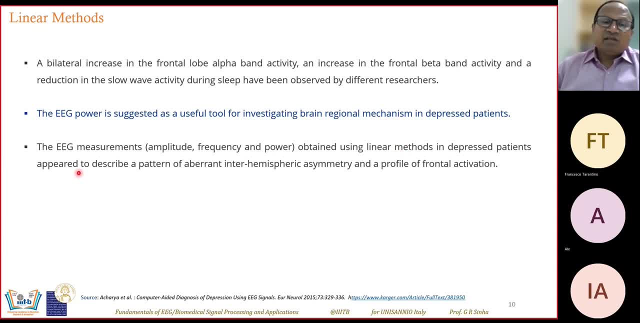 using the linear methods, even in the patients suffering with the depression, which helps in describing the brain regional mechanism. So we can use the linear method to study the brain regional mechanism. So we can use the linear method to study the brain regional mechanism. So we can use the. 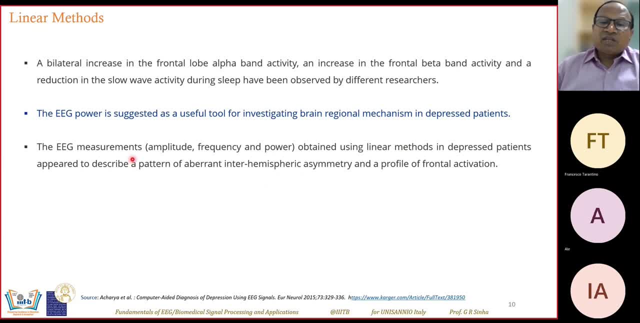 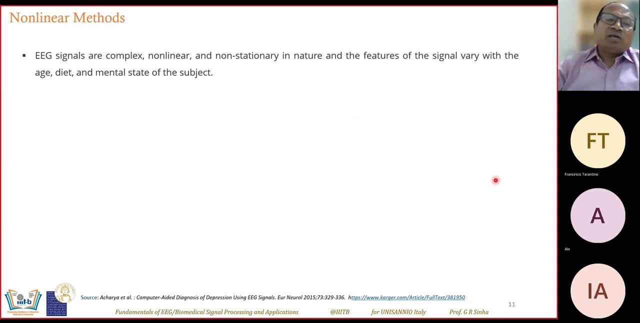 pattern of aberrant interhemispheric asymmetry in the EEG signal with a profile of frontal activation. Similarly, the nonlinear methods, which are much better than the linear methods. We know that the features are very important to understand the disability and we also know that EEG is a complex 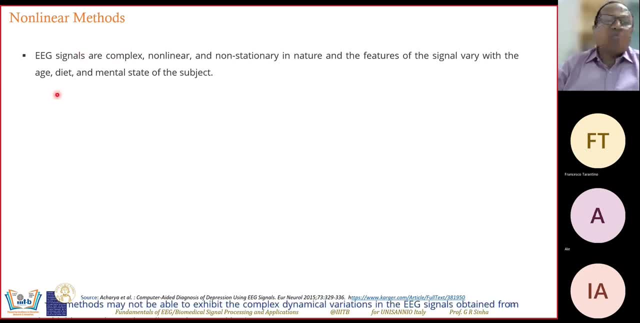 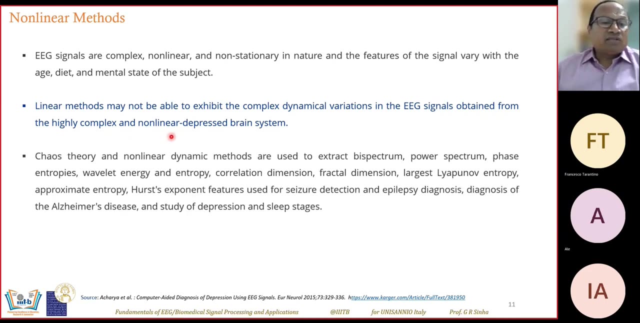 in nature. So therefore the nonlinear methods can actually help in understanding the problem more you know deeply Linear methods may not be able to exhibit complex dynamic variations obtained from the highly complex and nonlinear depressed brain system. So there are some examples: chaos theory and nonlinear dynamic methods are used to extract bispectrum like 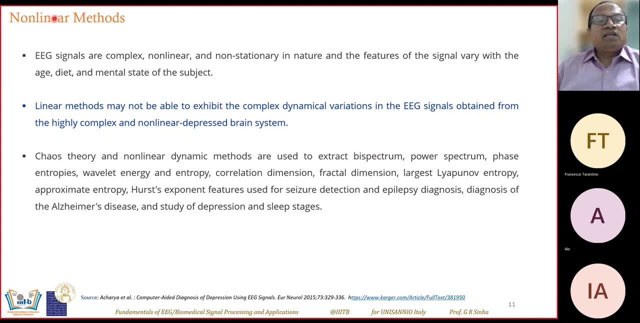 amplitude, frequency and power are calculated simply in a linear method. but in nonlinear method there are more number of attributes or features which can be determined, like extract, bispectrum, power, spectrum, phase entropy, weibullet, energy entropy, correlation dimension, fractal dimension, largest. 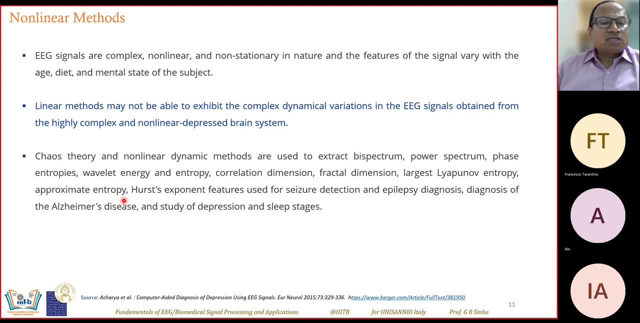 weibullet entropy, approximate entropy, host exponent features. All these new parameters or features which are extracted with the help of nonlinear methods are used for seizure detection, epilepsy diagnosis. You know that. what is seizure and what is epilepsy, we have covered in previous. 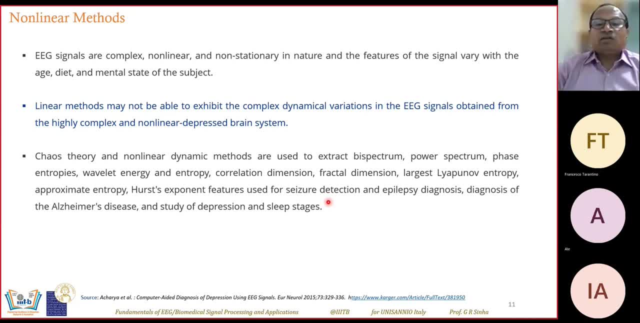 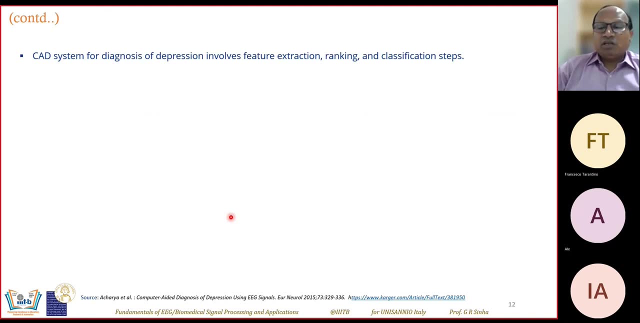 lectures that these are extremely, you know, severe disorder in terms of the brain functioning, the diagnosis of Alzheimer's disease and study of depression and study of even the sleep stages. All these are, you know, done more accurately, in a better way, by using nonlinear method, CAD system for diagnosis of depression. when we want to plan, 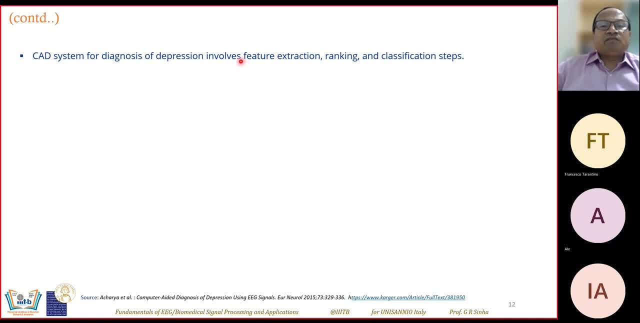 we want to implement CAD for depression. that involves feature extraction, ranking and classification. Different nonlinear methods can be used to extract the features. I think some examples are there, which are: fractal dimension, recurrent quantification analysis, higher order spectra, sample entropy, approximate entropy, largest Lyapunov exponent. 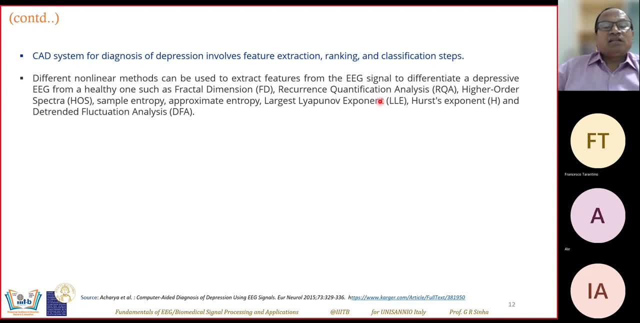 host exponent: detrended fluctuation analysis. These are some metrics and what we have done with this is to use the methods which are used in CAD system as the nonlinear approaches to better understand and better, you know, analyze the, the signal, And then which feature is more important. If you remember, in one of my previous lecture, 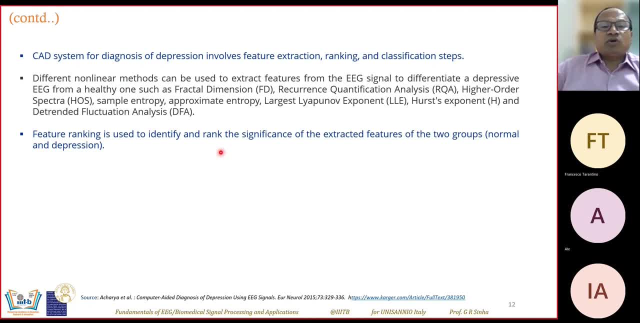 I talked about a ranking method that helps to rank either a method or a feature. So feature ranking is used to identify the rank and significance of appropriate features of the two groups. abnormal person who is suffering with, you know, depression. So student t-test. there is one t-test. 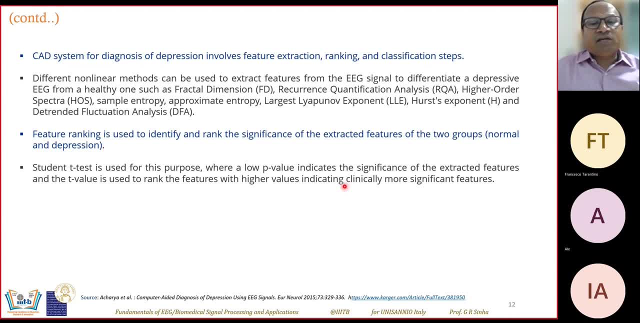 which is very popularly done for that assessment, where a low p-value indicates significance of appropriate features and the t-value is used to rank the features. So p-value indicates the significant, how important the features are, where t-value is used to indicate the rank of. 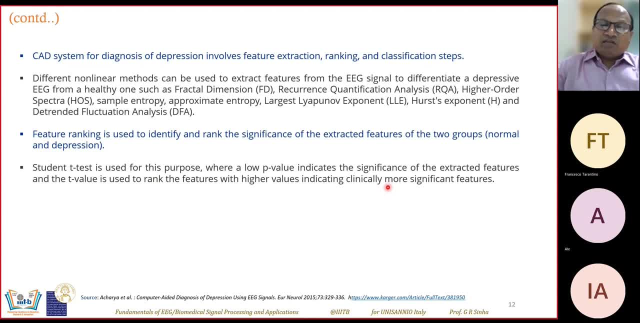 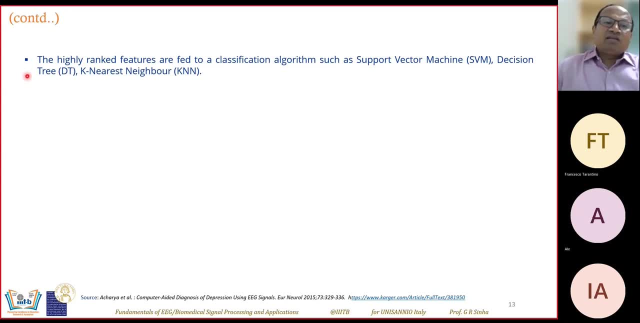 features with higher values indicating clinically more significant features. Highly ranked features are then given as the input to classifiers such as SVM decision trees or k-nearest neighbors, because we are choosing most appropriate and most highly ranked features so that can also help us in reducing the, you know, computational complexity as well as. 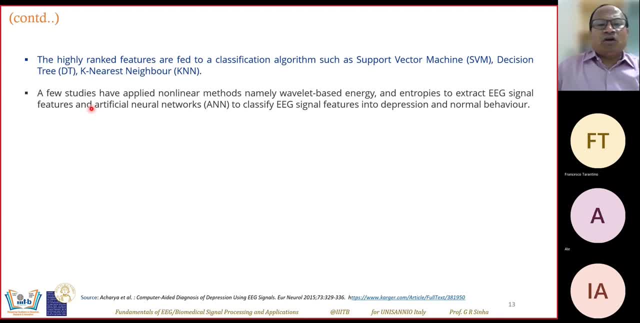 reducing the processing time. So there are studies which report nonlinear methods of the process and they are very good at that. So there are studies which report nonlinear methods like wavelet-based energy method and tropies to extract EEG signal using ANN and other methods. 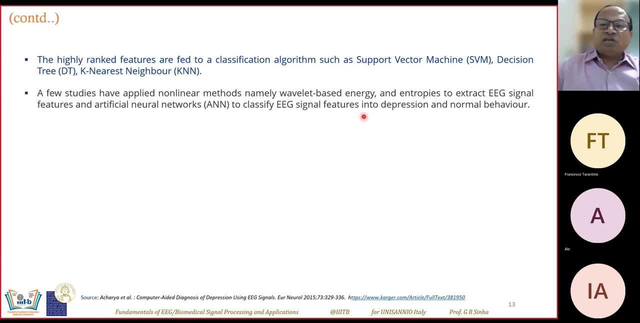 that can help to classify the depression behavior with the normal behavior. The frontal lobes of the brain, left and right, are compared in EEG full band and subbands with the goal of discovering relevant features. The enhanced probabilistic neural network, EPNN, is also used to differentiate. 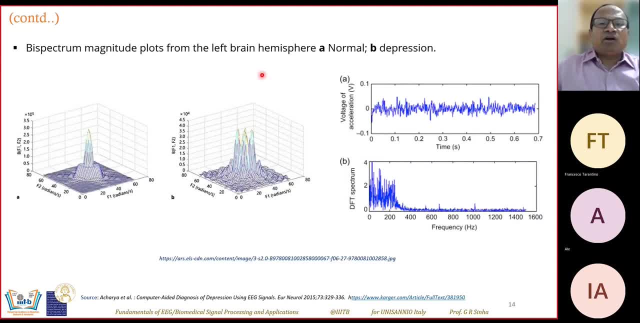 healthy EEGs. So this is the bias spectrum magnitude plot for the normal person in case in A and in the B it is for depression. you know stage And the same has been plotted. that is the first one is the amplitude response. 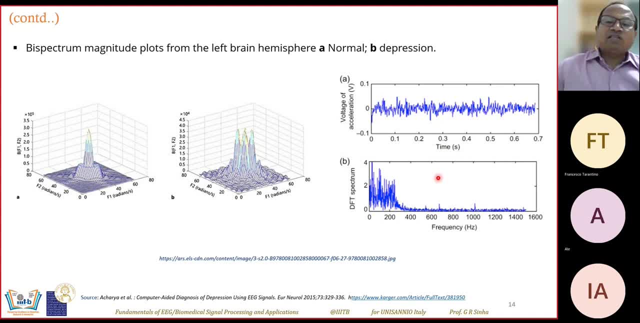 spectrum and the second one is actually the frequency response, where the DFT is plotted versus frequency. And these tools can be, you know, can be used to study the, you know, the depression like in left brain hemisphere. the bias spectrum is a tool, the 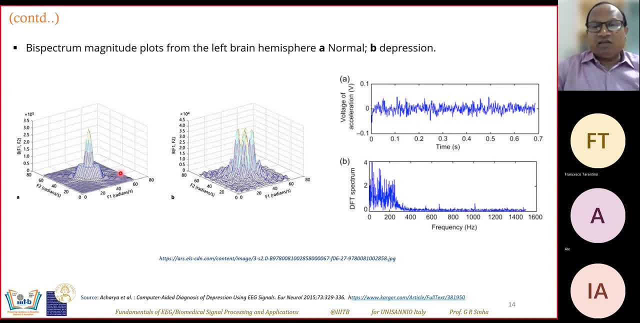 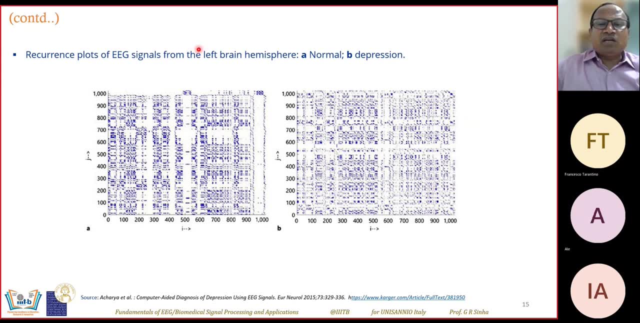 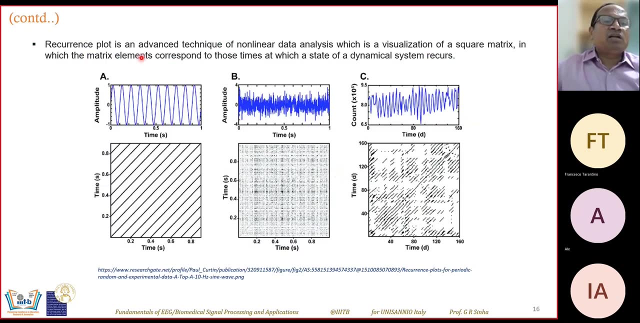 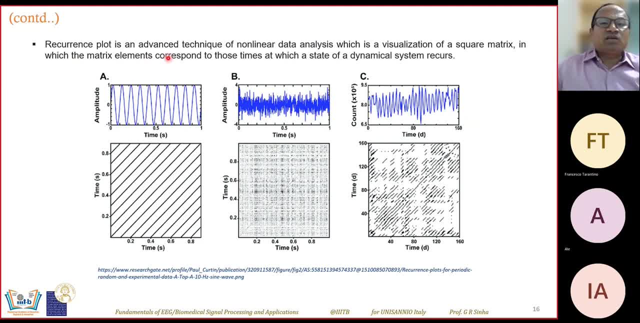 you will see lots of squares there in which the matrix element corresponds to those at each state of dynamic sistem occur. So each is square will represent something: Dimem, Acceleration, Neuter Missile. Each to square will represent some dynamic mental activity, Symptoms, Life quality. 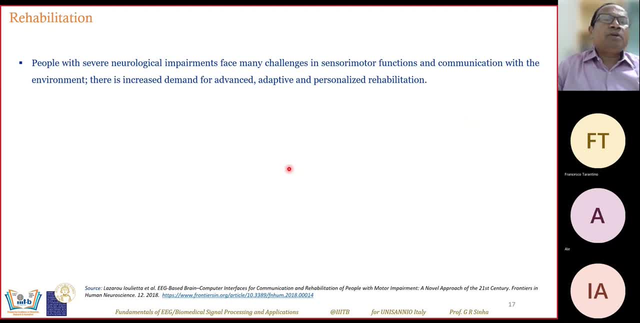 Talking about rehabilitation, people with severe neurological impairments in agriculture, 건강, pilot research and lineage are character abilities. they actually face many challenges in sensorometer, sensory motor functions. they are unable to move, they are unable to, you know, connect with the motory task with their sensor input and and 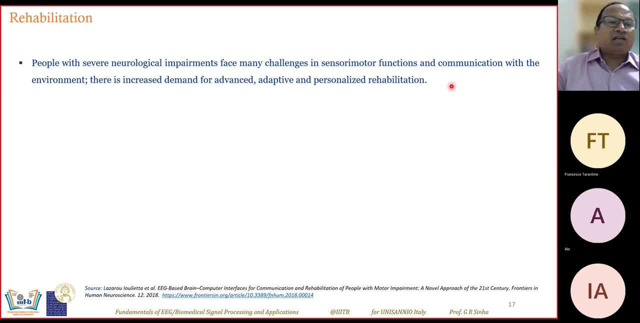 communication also they are. you know they have difficulty in communicating with the outside world. an increased demand for therefore advanced adaptive and such kind of rehabilitation technique is there. so studies have developed a number of bcis that aims are providing means of communication to the functional rehabilitation. ongoing research on non-invasive eeg based bci that can help in 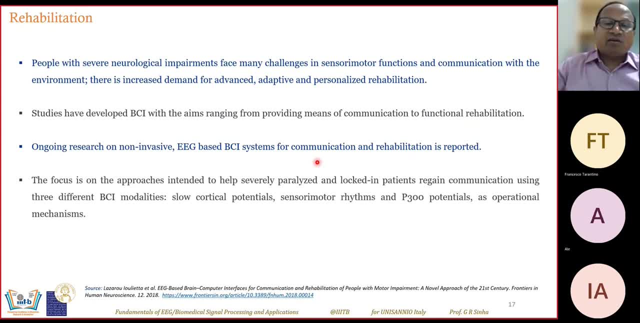 enhancing the communication so that the rehabilitation can help the people who are either in the old age or having certain disability. so the emphasis is on to develop the approaches that can help see the in the old age or having certain disability. so the emphasis is on to develop the approaches. 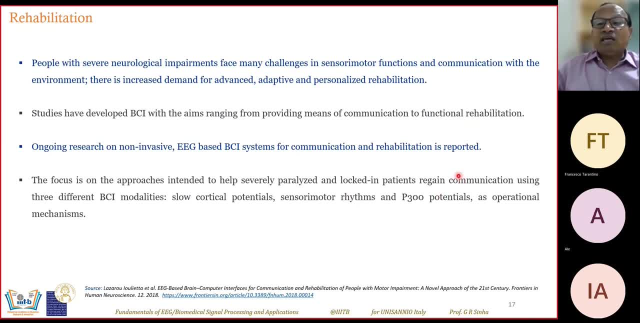 paralyzed, locked in, patients who can regain communication using three different bci modalities: either slow cortical potentials, sensory motor rhythms- we call it as smr- and p300 potentials as operational mechanisms. so these are the mechanisms or the modalities which are used in rehabilitating the patients who have been severely paralyzed or or suffering with severe 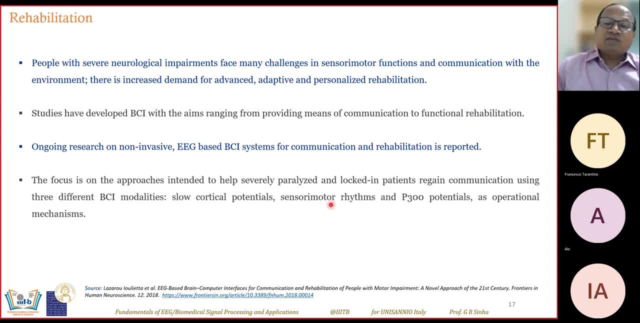 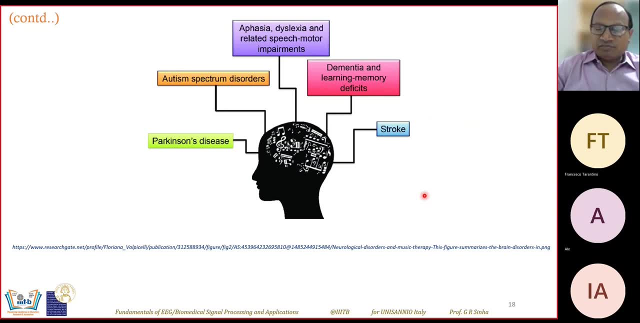 disabilities: slow cortical potentials, sensory motor rhythms and p300 potential. we have had enough discussion on p300. you know potential. so this is one example that indicates the severe disabilities related to stroke and parkinson's disease, autism spectrum disorder, dementia and learning memory deficit. dementia is something 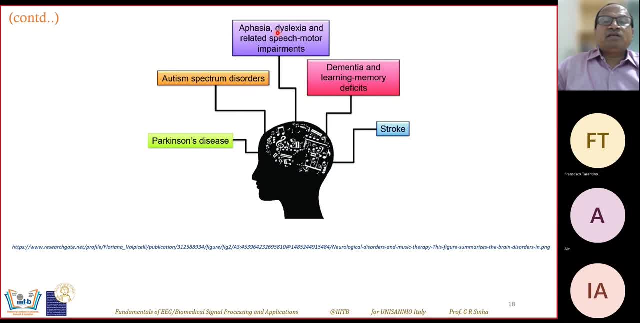 where the loss of memory is affects the person. aphasia, i mean dyslexia and related dyslexia and speech disorder. motor impairment is there. that is actually, you know, that belongs to this particular part of the brain. so there are. this diagram is actually indicating the severe disorders and 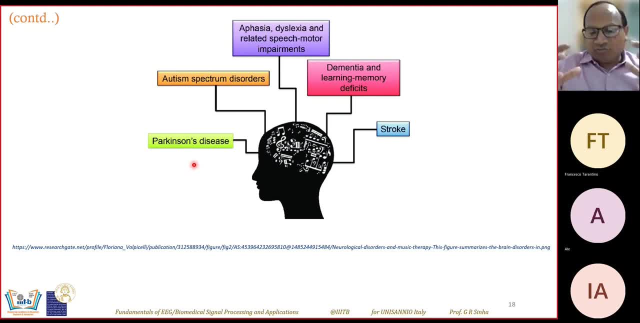 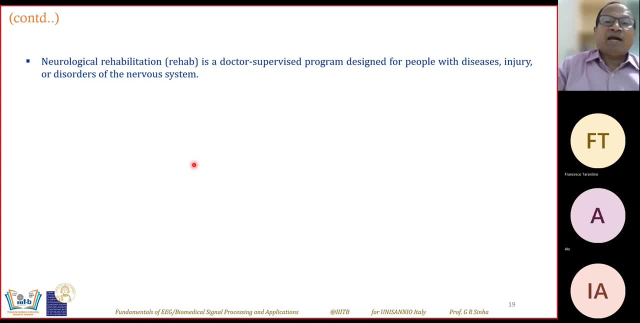 disabilities in terms of sensory motor. you know activities and sensory motor functions of a person. so neurological rehabilitation, called as rehab, is a doctor supervised program which is designed for people with diseases, injury or disorders of nervous system. so this is a diagram that indicates neurological rehab can often improve functionality, can also reduce symptoms and improve the well-being. 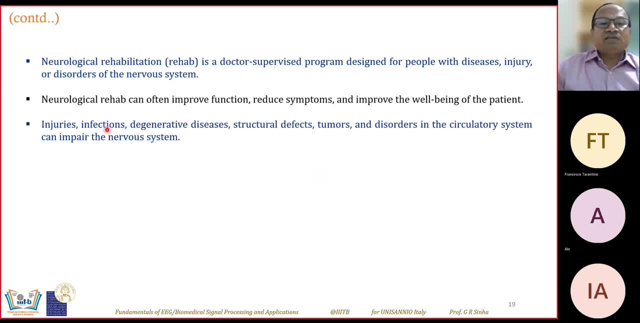 of the person who is suffering. injuries, infections, degenerative diseases, structural defects, tumors and disorders in circulatory systems can impair the nervous system. the vascular disorder, such as, uh, you know, ischemic strokes caused by blood clots, and then there is another term called as hemorrhagic strokes caused by bleeding in the brain, then subdural hemo hematoma, and transient 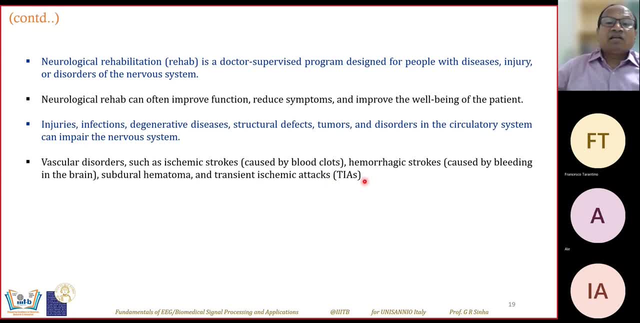 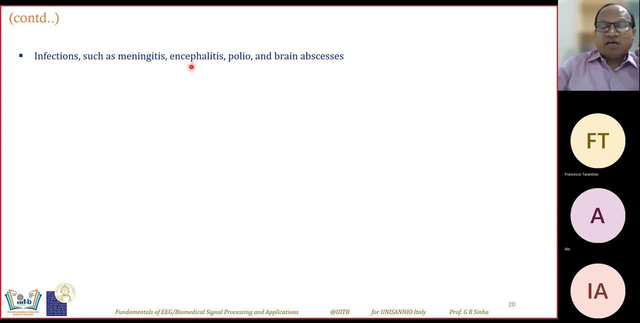 uh, ischemic, ischemic attacks, that is, tias. so these are the severe, you know difficulties: trauma such as brain and spinal cord injury, uh, and infections such as, you know, encephalitis, polio, brain abysses, structural neuromuscular disorders such as bale. 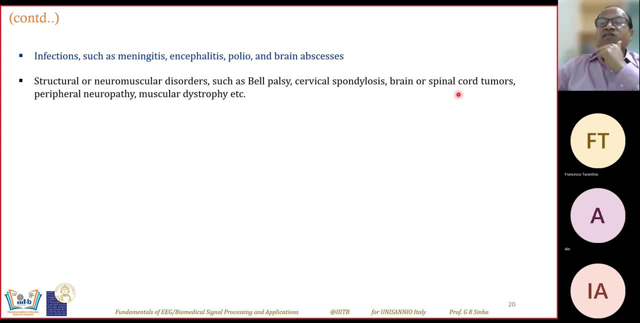 palsy, uh, you know. cervical spondylitis, brain and spinal cord tumors, peripheral neuropathy, muscular dystrophy, etc. functional disorders such as headache, seizure disorder, dizziness and neuralgia. degenerative disorders: disorders include parkinson's disease, multiple sclerosis and amotropic lateral sclerosis, called as als and alzheimer's disease. so this diagram is not 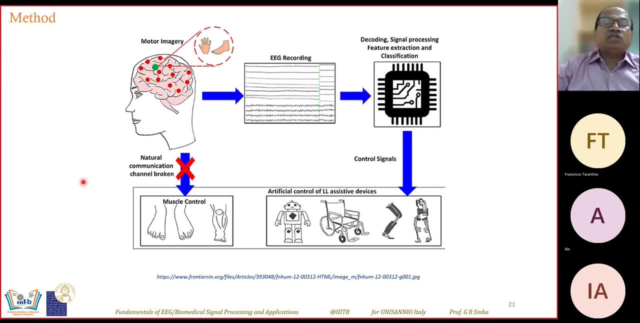 uh, you know, you know a new diagram- we have used this kind of picture in all our previous lectures- that how do we uh use the rehabilitation uh to cure a person, to reverse the disorder or disability where the imagery is captured, eeg is recorded, then we decode, we apply suitable electronic circuit. 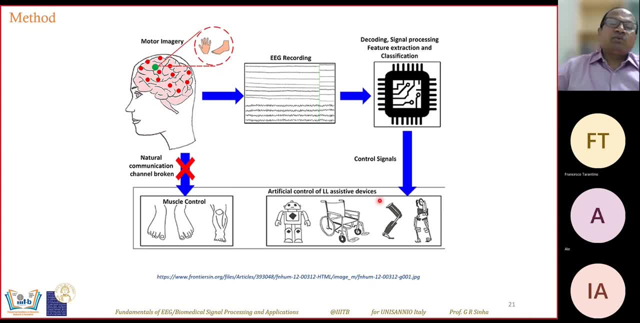 signal processing, feature extraction, classification, then either we generate some control signal signals that can be either artificial, intelligent controlled vehicles or, you know, bci controlled wheelchairs, or robotic arms, robotic legs, etc. and even the robot can help the person to you know to, to bring it to some normalcy, or some kind of feedback signals are given to the person. 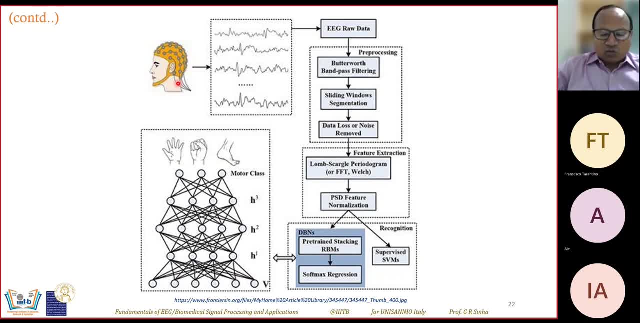 and the rehabilitation is done. so this is one such example of you know. we can see a flow diagram where eeg is recorded, raw data, and these are the all ordinary stages. see, in the pre-processing a butter worth bandpass filter is used, butterworth message. these are the standard filters function, then sliding window segmentation is applied. so 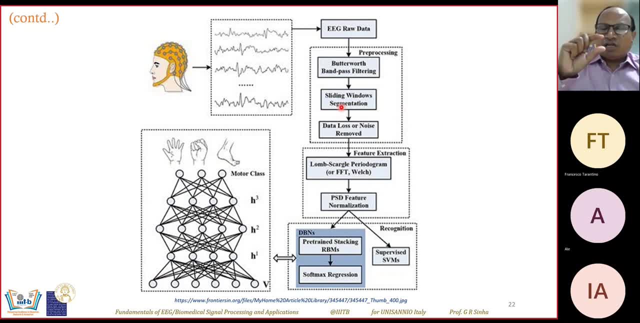 that suitable. you know that band of signal could be chosen and the data laws are noise. if there is some data loss that can be recovered, we can apply that to the disease or the noise is there in these process. then noise can be removed and then we can use fft or welch. 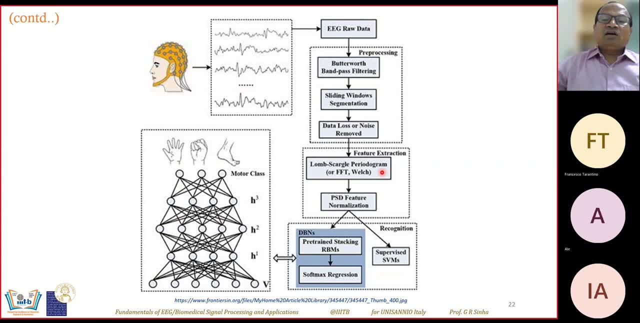 well you know, weblet based method to determine the uh, the number of features, and we can calculate psd feature or any other feature and apply the normalization. then we can use any suitable method for classification and then that classification output can generate either the feedback signal. 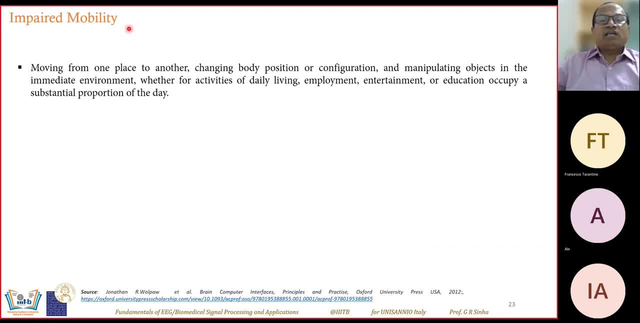 of the command. so moving from. like impaired mobility, person is unable to move, moving from one place to another, changing body position or configuration and manipulating objects in immediate environment, whether for activities, daily living, employment or entertainment, or education. that occupies substantial proportion of the day where we need mobility. so number of diseases and 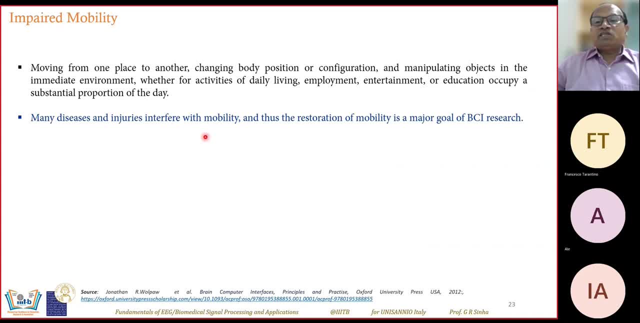 injuries interfere with mobility and therefore restoration of mobility is a major problem in the goal of bci research, where, if you can- uh you know- achieve some mobility in the patients, so with the mobility, many other problems, many other uh you know things, uh the disabilities could be recovered. to begin with, we need to recover the mobility, so therefore it's important. 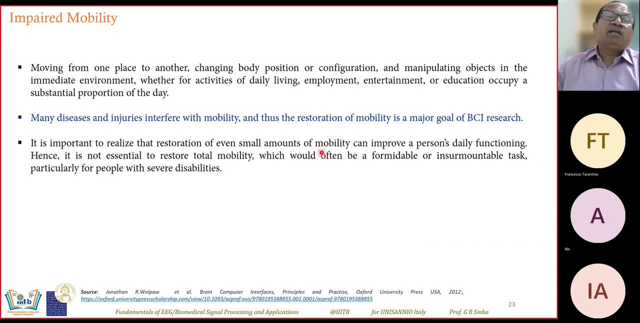 to realize a restoration of even a small amount of mobility, if you are even able to move a very small amount of mobility which can improve the person's daily functioning- and it's not essential to restore total mobility, but slight restoration of mobility can also be helpful- and, uh, you know- so that a person can perform a slowly certain tasks and functionalities. 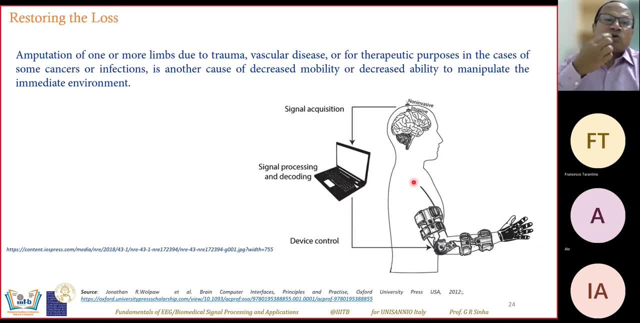 even the person who is having a severe disability. so, restoring the loss. like you see here, the signal processing is there and with the help of device control you can, you know, restore the movement. uh, like amputation of one or more limbs due to trauma, vascular disease or therapeutic purposes in the cases of some cancer or infection. 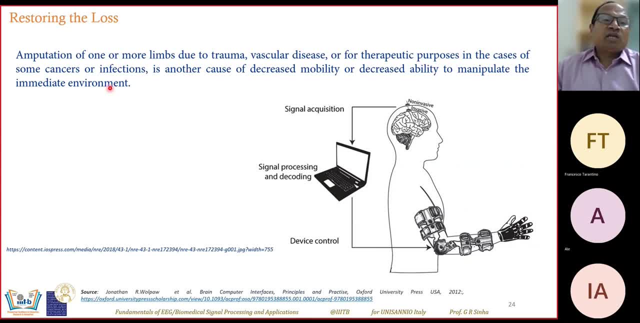 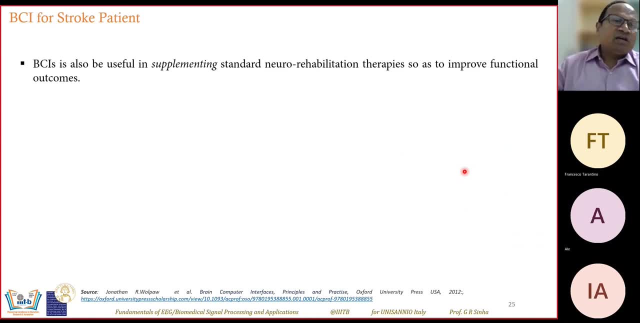 is another cause of decreased mobility or decreased ability to manipulate the immediate environment. so this could be, uh, you know the. the restoration of mobility could be achieved and, as far as the stroke patient is concerned, bci we have seen is used to supplement, augment, restore, if you remember. a number of functionalities are there, so one of the 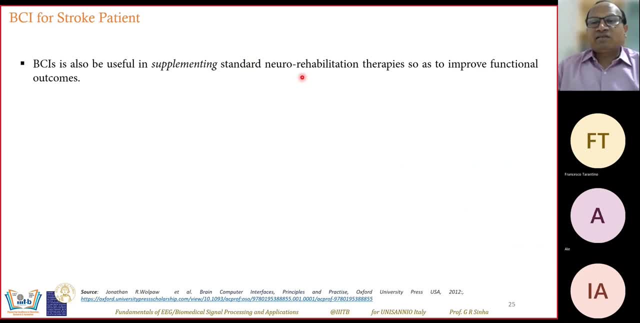 functionality is. supplement is a standard neuro rehabilitation therapy to improve the functional outcome and provide the recovery. physical, occupational, speech and language therapy, either physically or occupationally. or speech, you know, to say something in his ear or to you know convey some language, particular language, to the person. so these are the therapies which are commonly used in 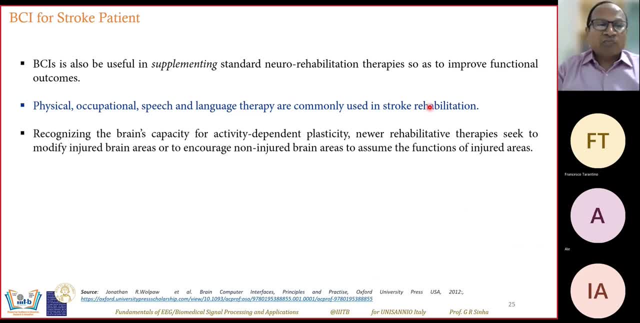 the rehabilitation of persons who are suffering with the stroke, recognizing the brain's capacity, activity dependent plasticity. newer rehabilitation therapies. sick to modify injured brain brain areas are encouraged. non-injured brain areas to assume functions of injured areas. bci is also contribute by encouraging the return of brain activity that can enable voluntary control of limbs and also. 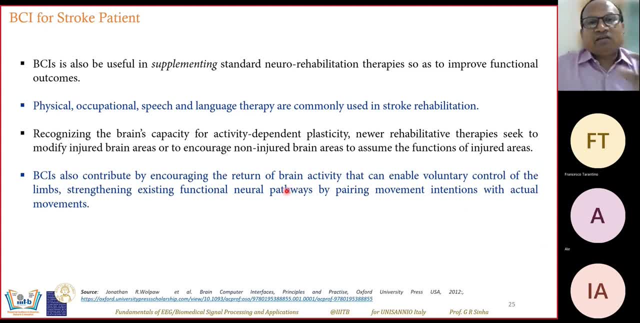 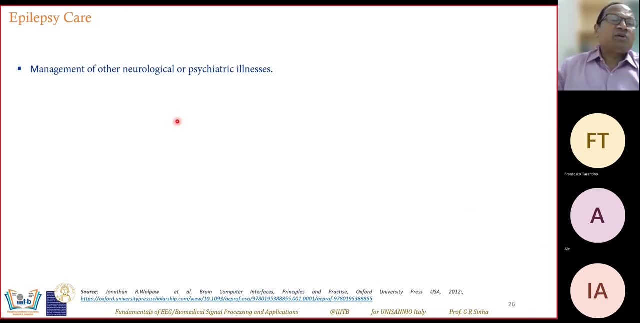 strengthen the functional neural pathways. uh, that has, you know, created the problem for mobility. so that can, uh, you know, provide some pathway to improve the function of the brain. so that can, you know, provide some pathway by pairing the movement intentions with the actual movement. next one is epilepsy care. the management of other neurological or psychiatric illness can also be. 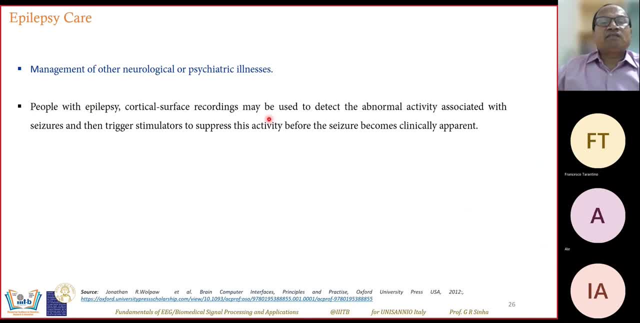 made possible. people with epilepsy: cortical surface recording uh are generally used. cortical surface recording scr can be used to detect the abnormal activities associated with seizures and trigger stimulators to suppress the activity or motor, desktop or physical activity. uh healing energy on those. Haha, yes, I had. 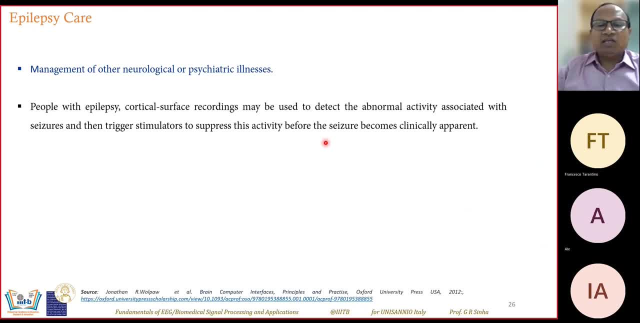 rheumatism. UPCI, PCS-E is a different thought primed that this is something that does carry to the yoga했ic: suppress the activity before seizures become clinically apparent. The system directly detects and affects the brain activities and such BCI can predict, impending you know, a seizure might. 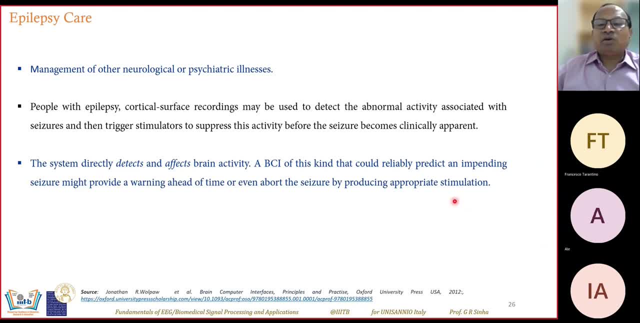 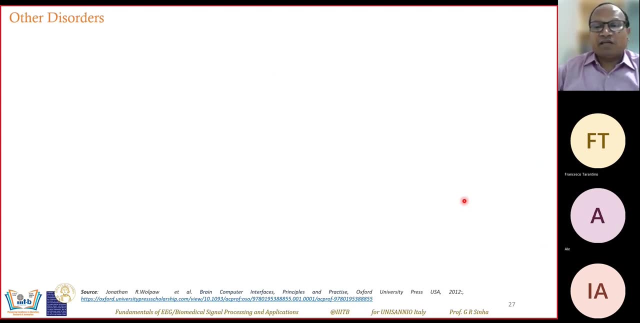 provide a warning ahead of time or even abort the seizure by producing appropriate stimulation. So either a warning can be generated or even it can be aborted, because seizures are very dangerous things. where there is a, you know, there might be loss of life directly. Other disorders are: 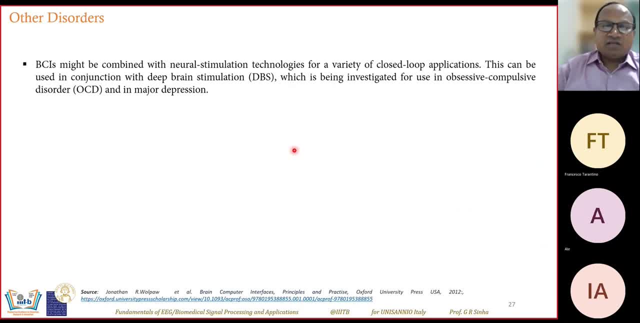 there, like there are some other disorders. BCIs might be combined with neural stimulation technologies for a variety of closed-loop application. You can understand what I mean to say by closed-loop application. Closed-loop application: you have a feedback, and this can be done in conjunction with deep brain stimulation, called as DBS. 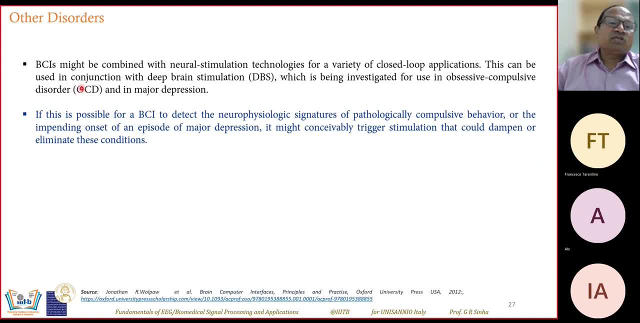 That is being investigated for use in obsessive-compulsive disorder and in major depression. So this kind of deep brain stimulation is recommended and, you know, investigated- rather a lot of still research is going on that can actually help the people with suffering with. 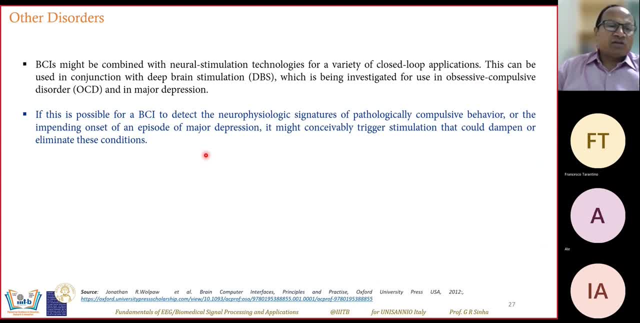 obsessive-compulsive disorder or the major depressive disorder. So if this is possible for a BCI to detect neurophysiologic signatures of pathologically-compulsive disorder, the impending onset of an episode of major depression, it might trigger the stimulation that could dampen and eliminate these conditions. So, getting the, you know the trigger and how. 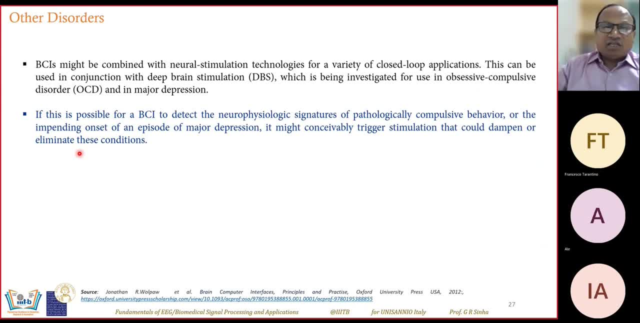 we will get the trigger, how we will decode the trigger? it is just because of deep brain stimulation is provided to the brain and we are trying to get the signal from there. So definitely the penetration and up to semi, at least up to semi-invasive level, we have to go.